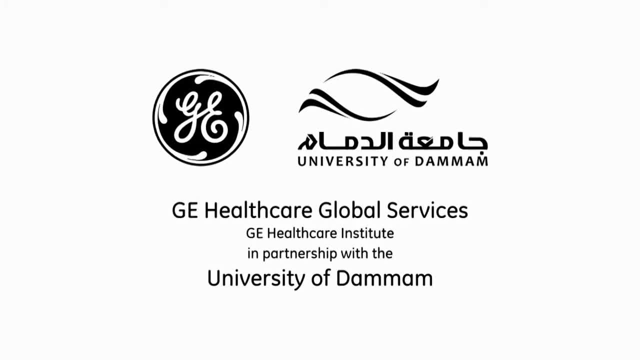 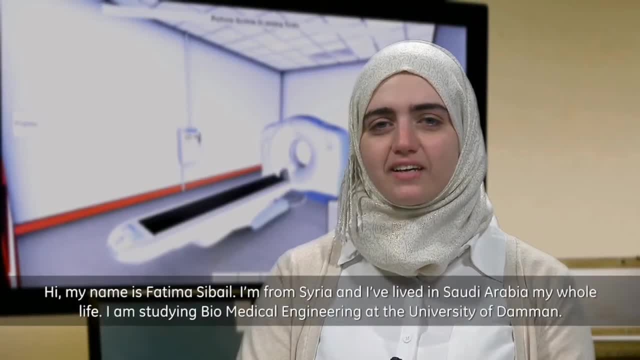 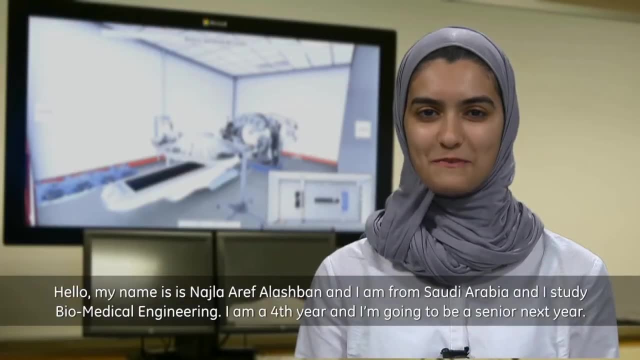 Hi, my name is Fatima Sibai. I'm from Syria and I've lived in Saudi my whole life. I'm studying biomedical engineering at the University of Dammam. Hello, my name is Najal Ashban. I'm from Saudi Arabia and I study biomedical engineering. 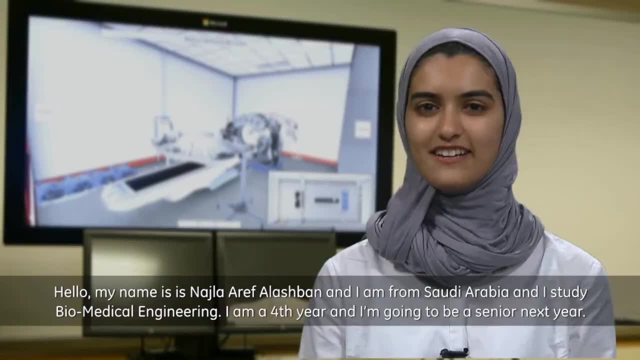 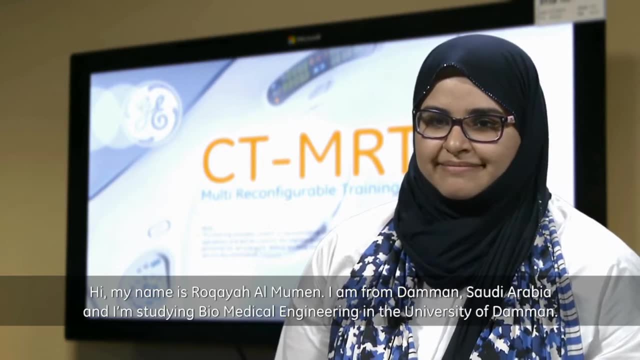 I'm a fourth year biomedical engineer. I'm going to be a senior next year. Hi, my name is Ruqayya Al-Muman. I'm from Dammam, Saudi Arabia. I'm studying biomedical engineering at the University of Dammam. 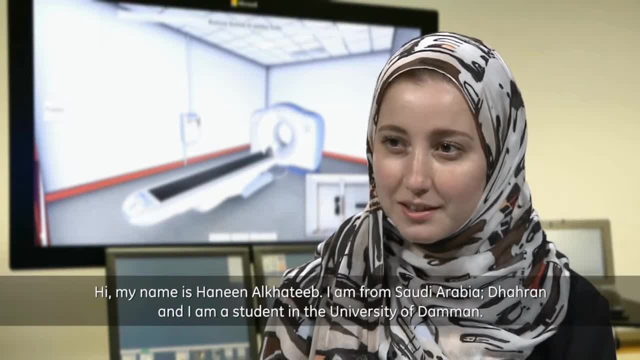 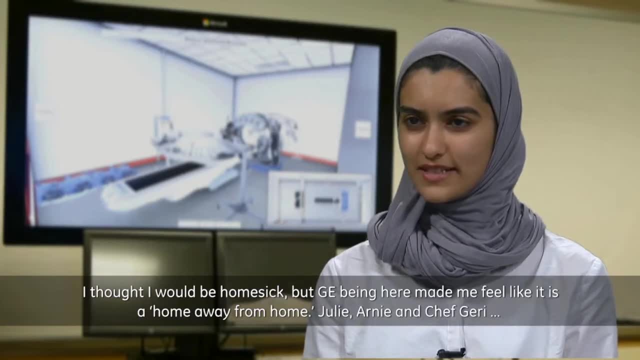 Hi, my name is Hanina Khatib. I'm from Saudi Arabia, Tehran, and I'm a student at the University of Dammam. I thought I would be homesick, but GE being here made me feel like I'm home, away from. 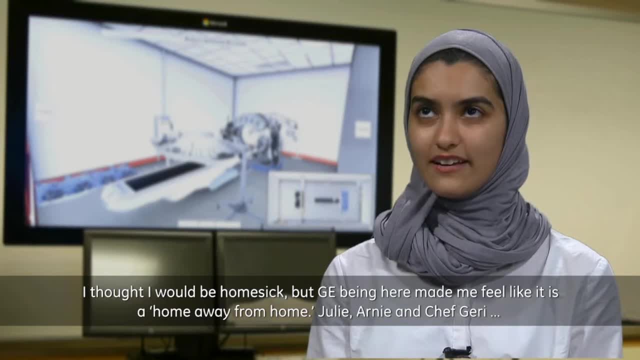 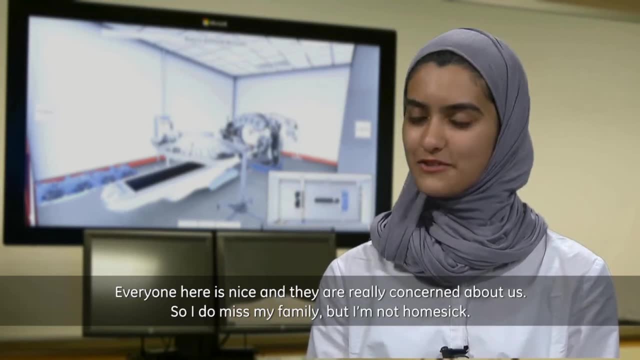 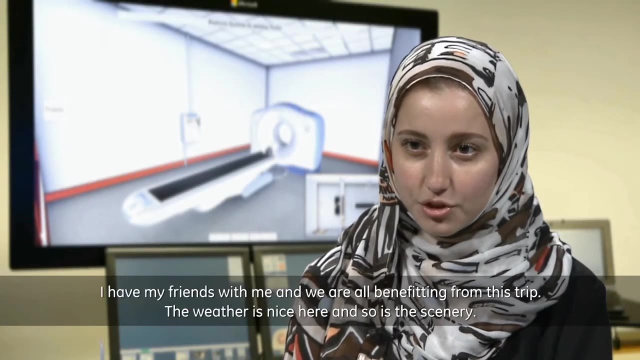 home: Julie, Arnie, Chef, Gary, everyone here is nice. They're really concerned about us. So I do miss my family, but I'm not homesick. I have my friends with me and we're all benefiting from this trip. The weather is nice here and 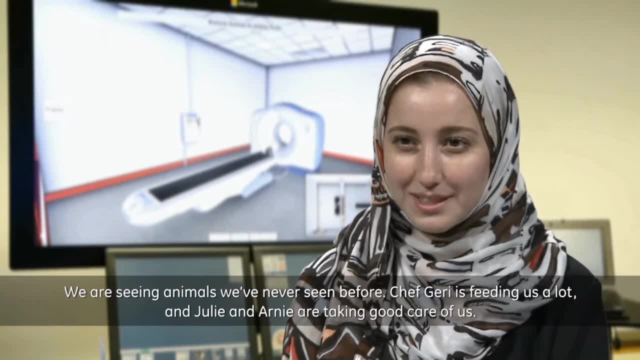 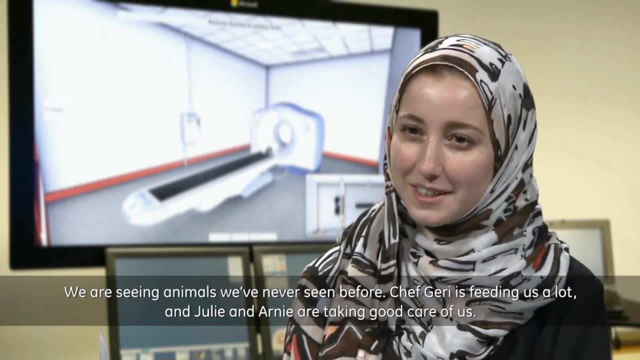 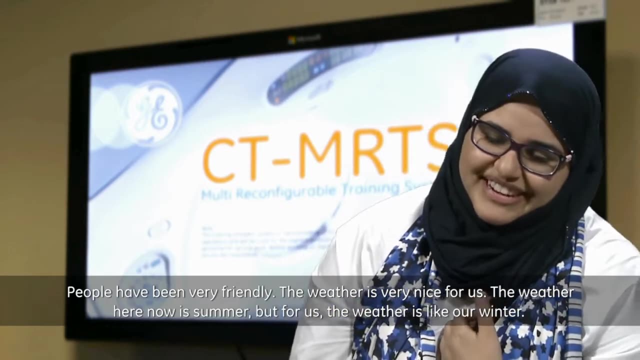 the scenery. we're seeing animals that we've never seen before. Chef Gary is feeding us a lot and Julie and Arnie are taking good care of us. People here are very friendly. The weather is very nice for us. The weather here now is summer, but for us this is the. 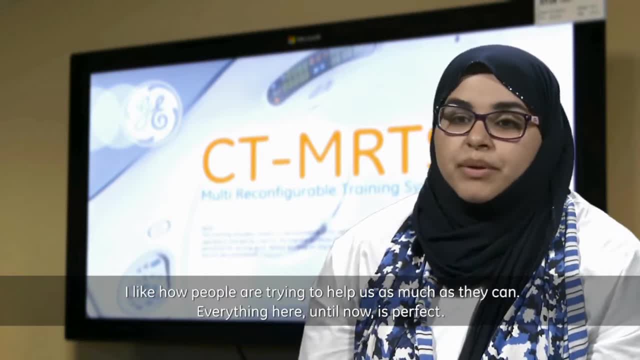 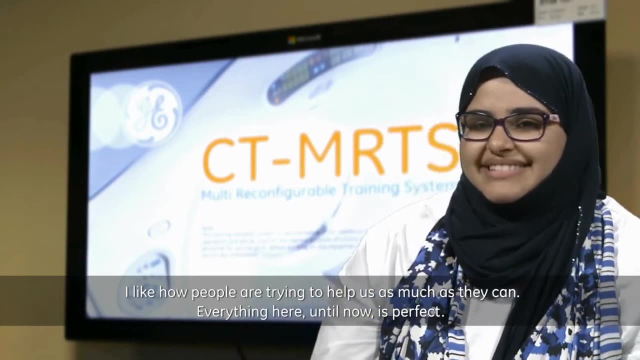 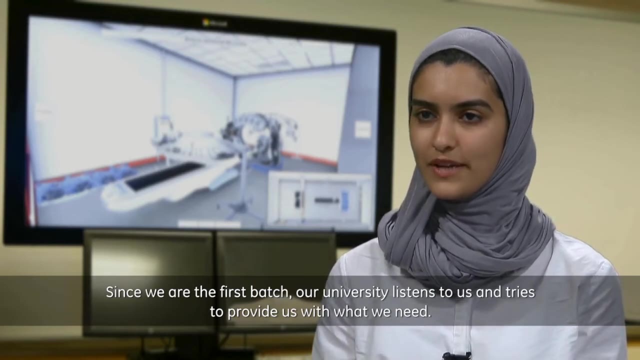 weather for us in the winter. I like how people are trying to help us as much as they can. Everything here until now is perfect, Since we're the first batch. our university listens to us and tries to provide us with what we need, And they recognize our potential and help us to work on it, And they they're. 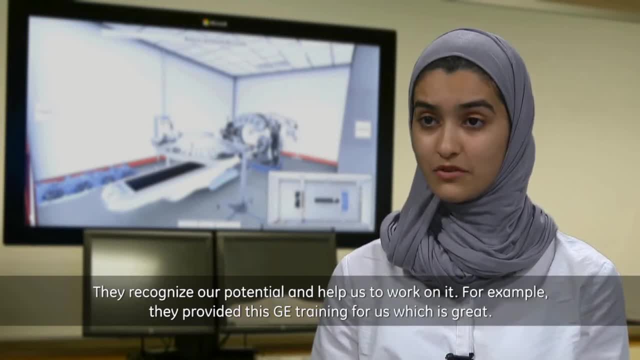 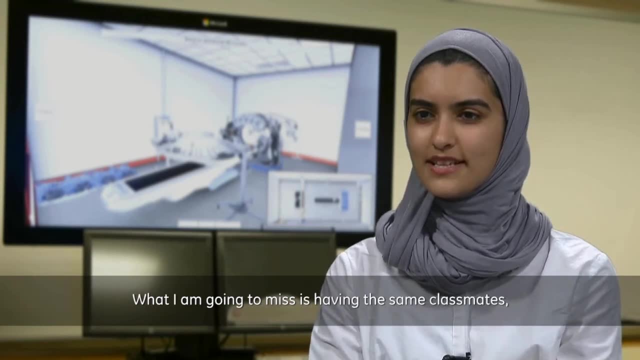 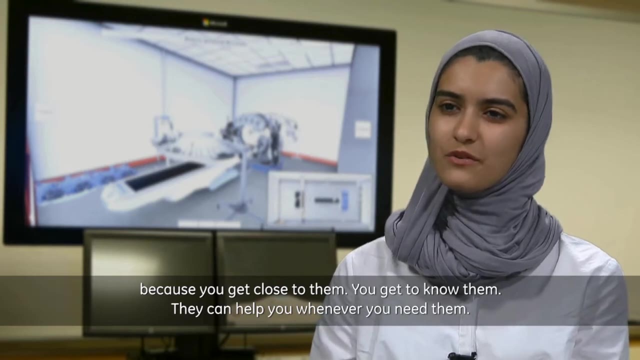 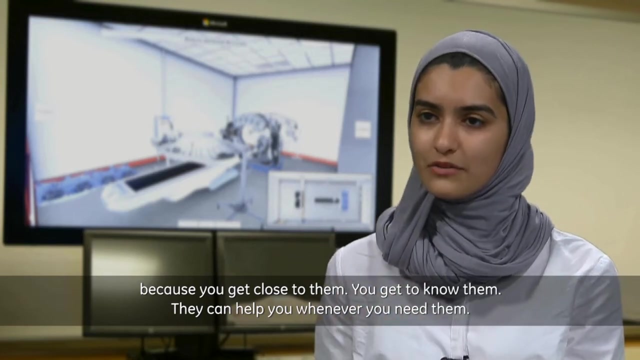 For example, they provided this GE training for us, which is so great and it's really great. What I'm going to miss is having the same classmates, because you get closer to them, you get to know them, you get to know that they can help you around whenever you need. 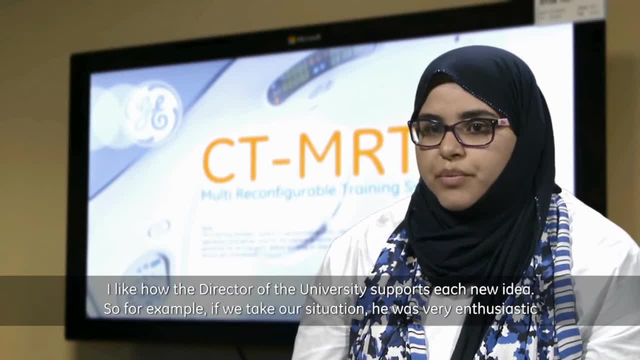 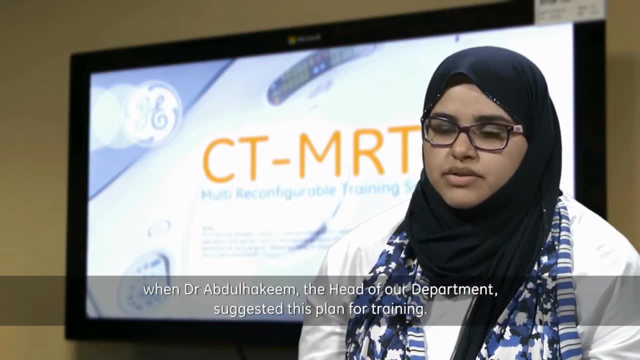 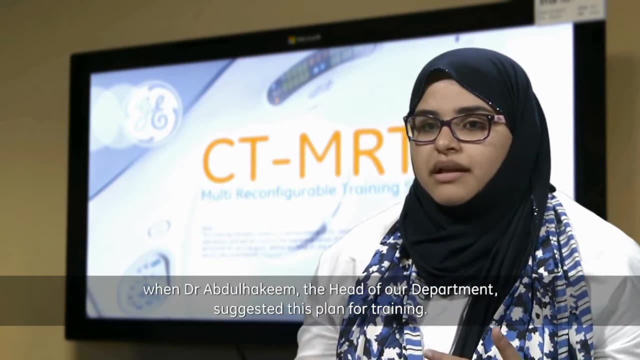 I like how the director of the university supports each new idea, Like, for example, if we take our situation, like he was very enthusiastic when Dr Abdul Hakim, the head of our department, suggested this plan for training Dr Abdul, who is the director. he was very supportive and enthusiastic for this idea. 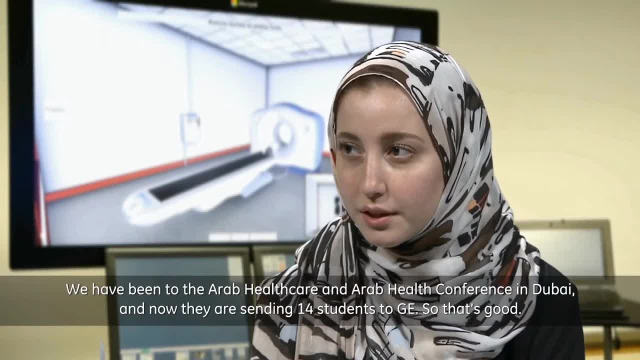 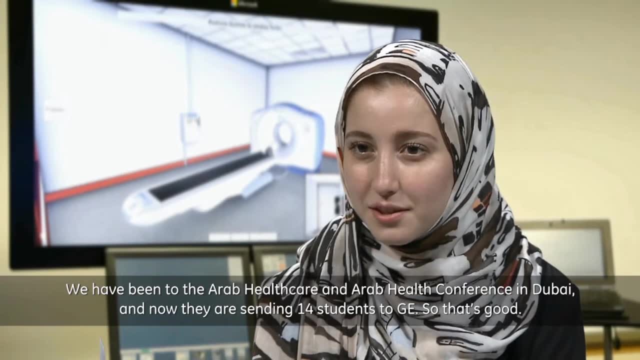 so I like how he supports this good idea. We've been to the Arab Health Care and the Arab Health Conference. We've been to Dubai and now they're sending 14 students to the GE. so that's good. yeah, It's amazing. 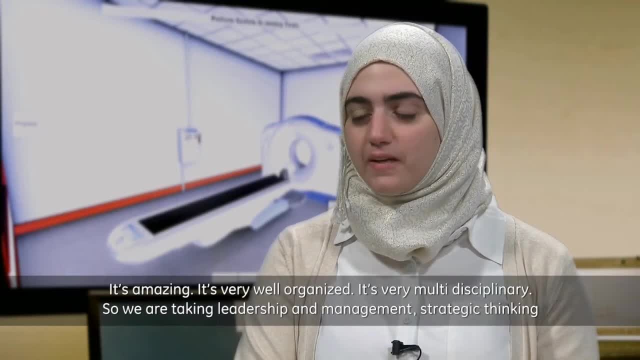 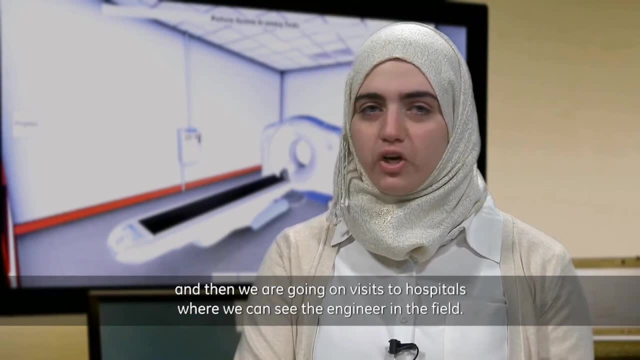 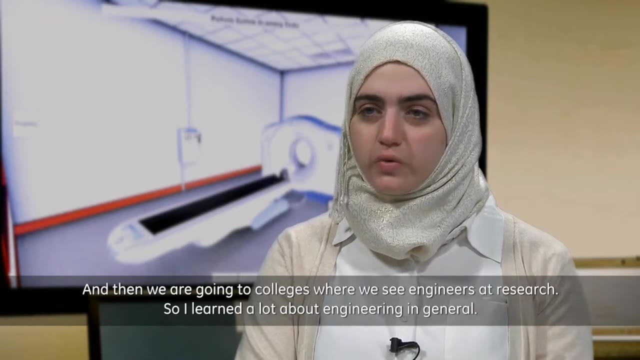 It's very well organized. I might say It's very multidisciplinary. so we're taking leadership and management and strategic thinking and then we're going visits to hospitals where you can see the engineer at the field, and then you go to the colleges where you see engineers at research. 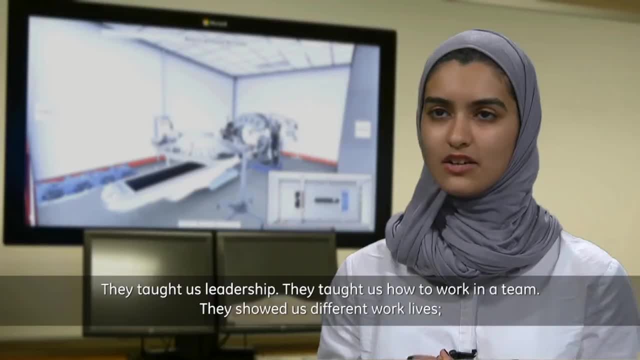 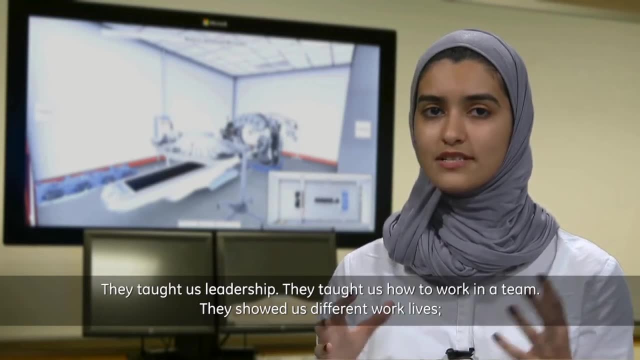 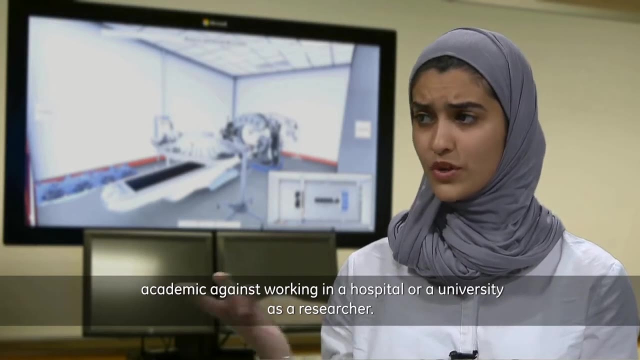 So I kind of like I learned a lot about engineering in general. They taught us leadership. they taught us how to work in a team. they showed us different work life- you know academics versus working in a hospital or in a university as a researcher. 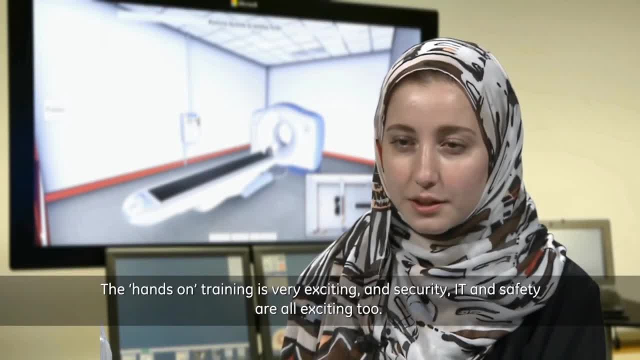 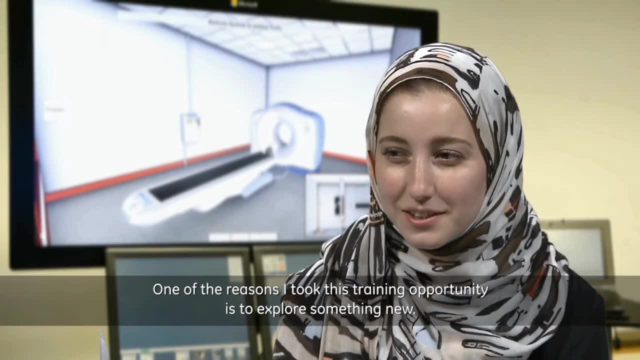 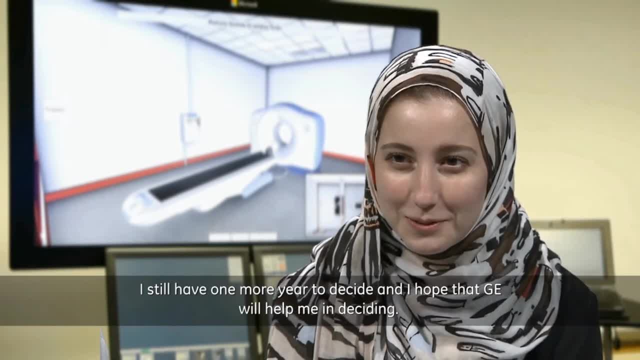 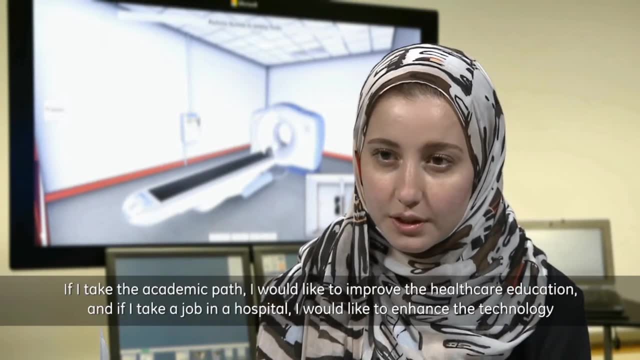 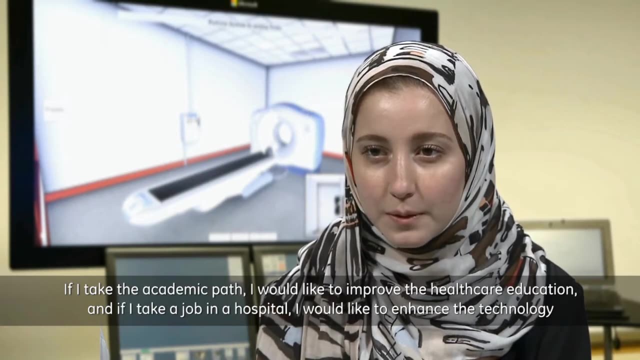 I still have one more year to decide and I hope that GE will help me in deciding. If I take the academic path, I would like to improve the education, the healthcare and the education, and if I take a job in a hospital, I would like to enhance the technology to. 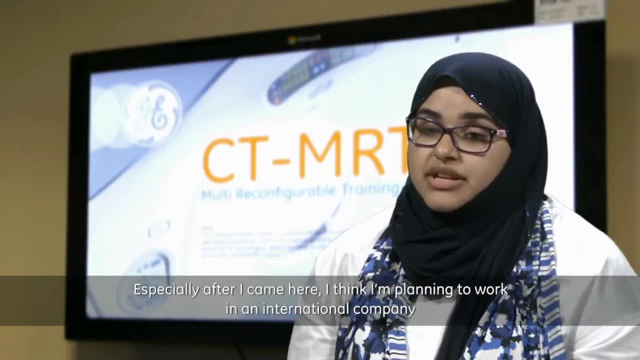 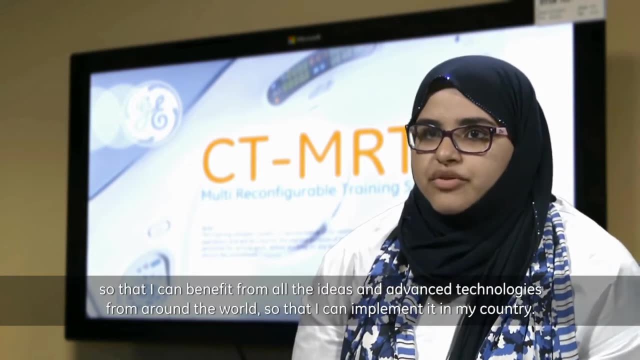 make it as advanced as we've seen here, Especially after I came here, like I think, I'm planning to work in an international company so I can benefit from all the idea and advanced technologies around the world so I can implement it in my country. 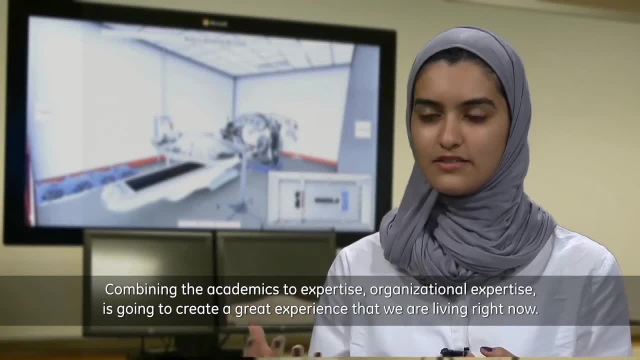 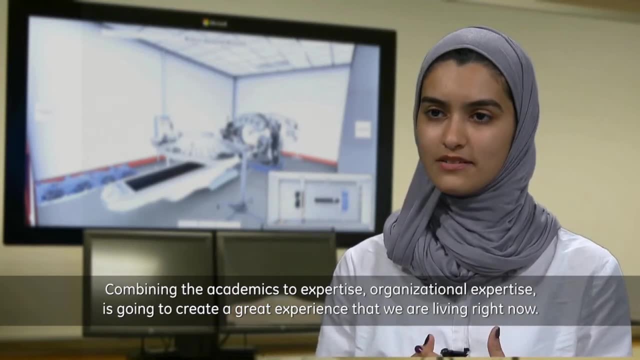 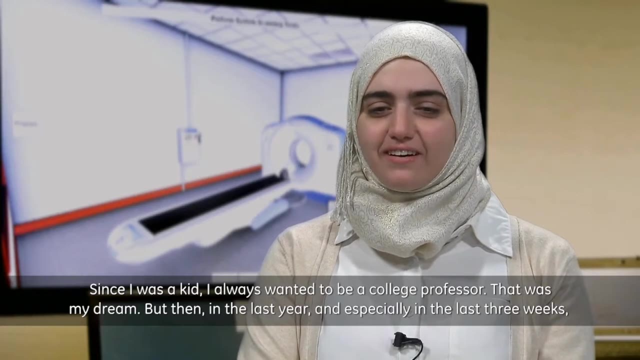 Combining the academics like academics to expertise, like organization expertise is going to create a great experience, just like what we're living right now. Since I was a kid, I've always wanted to be a college professor. That has been my dream. 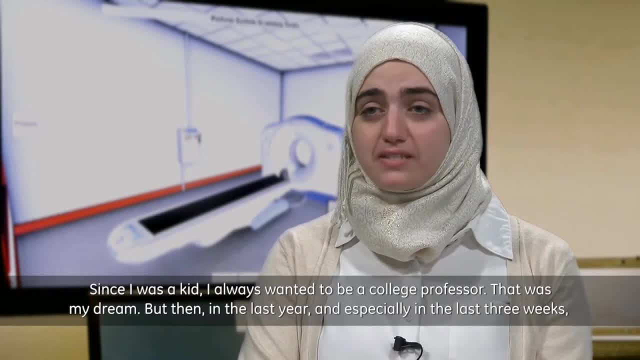 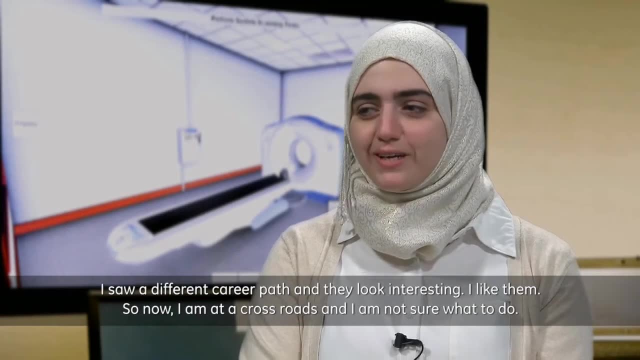 But then in the last year, and especially the last three weeks, I kind of saw the different career paths and they're interesting. I don't mind them, I like them. So now I'm kind of like at crossroads. 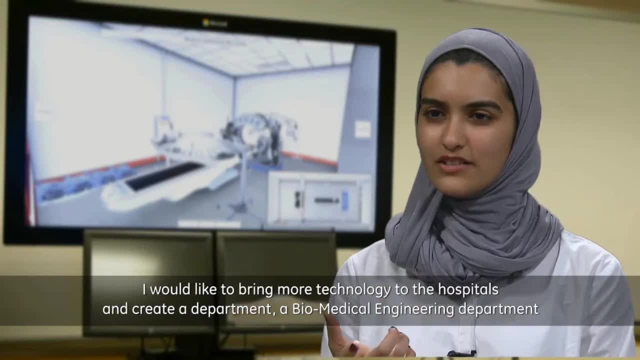 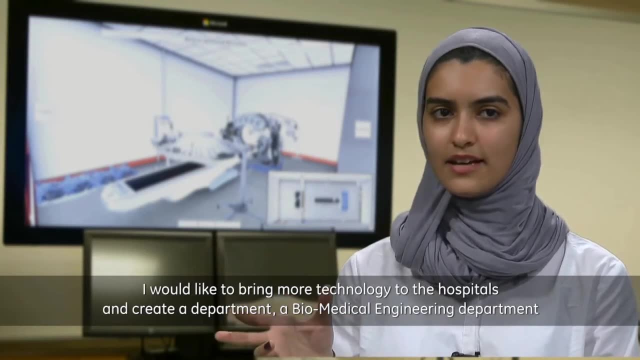 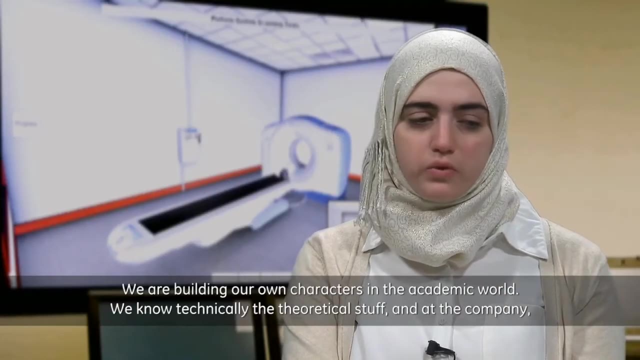 I'm not sure what to do. I'd like to bring more technology to the hospitals and create a department, a biomedical engineering department, that helps in doing those things, Implementing them. We're building our characters in the academic world. We know the technical, the theatrical stuff. 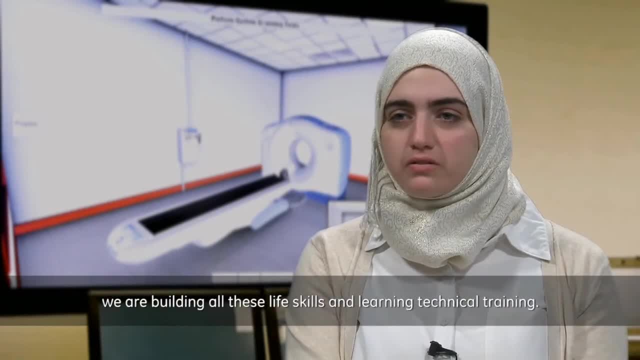 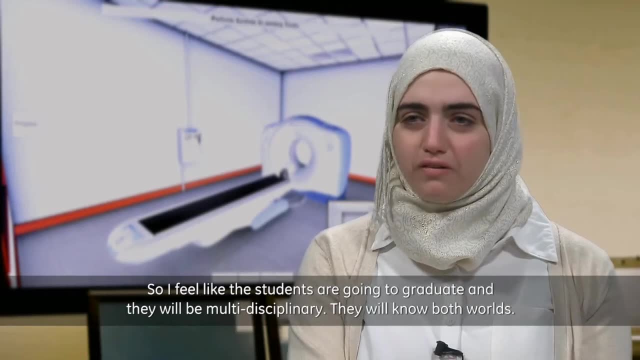 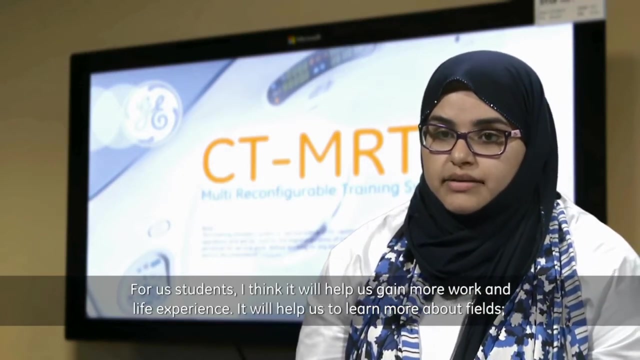 And then at the company we're building all those life skills and we're learning technical training. So I feel like the students are going to graduate and they will be multidisciplinary. They'll know from both worlds. you know, For us students, I think it will help us to gain more work and real-life experience. 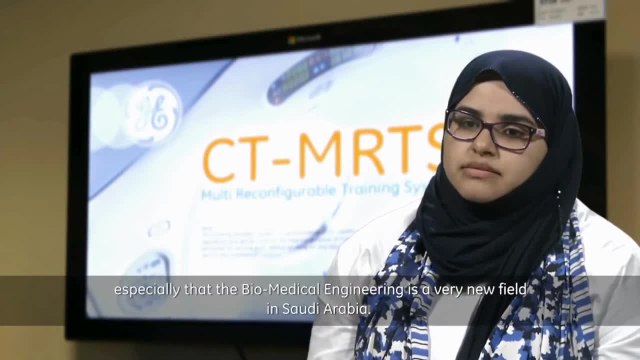 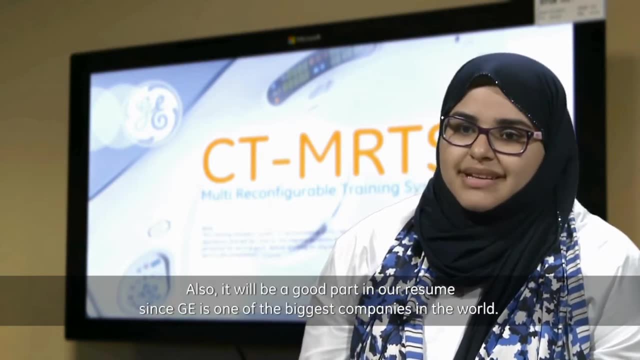 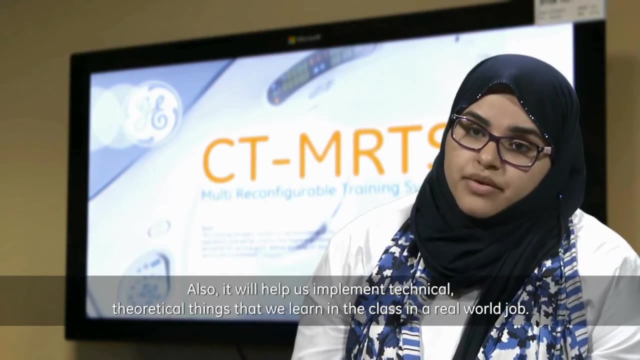 It will help us to learn more about fields, Especially that biomedical engineering. Biomedical engineering is a very new field in Saudi Arabia. Also, it will be a good part in our resume, since GE is one of the biggest companies around the world. It also will help us know how to implement the theoretical things that we learn in the 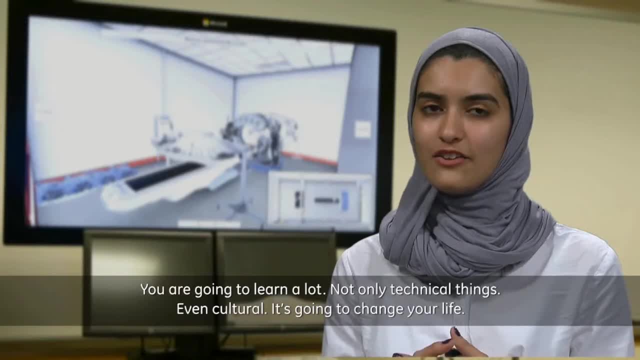 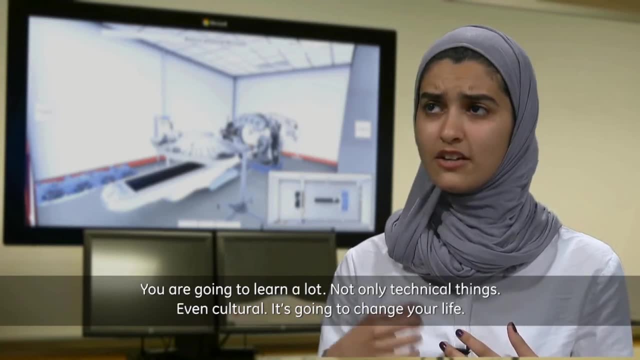 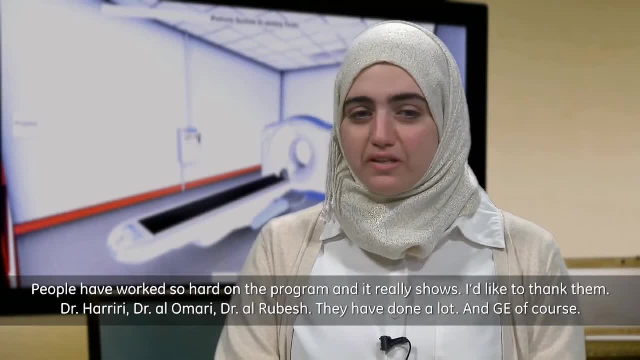 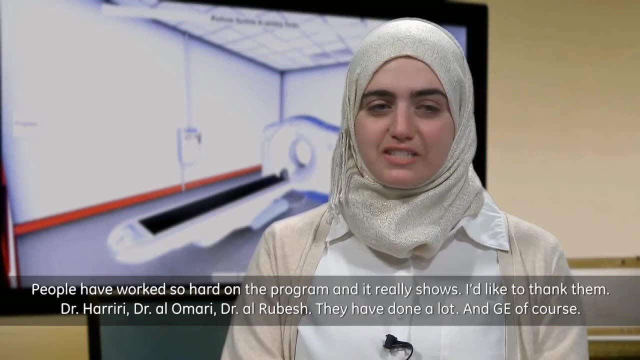 People have worked so hard on the program and it really shows. I would like to thank them: Dr Hariri, Dr Omari, Dr Rubesh- They've done a lot- And, of course, the GE. If given the opportunity, I encourage them to join. 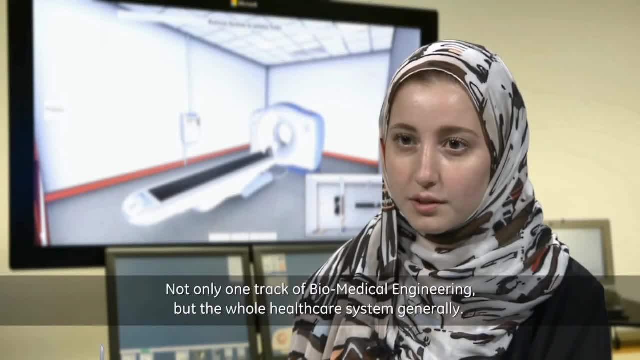 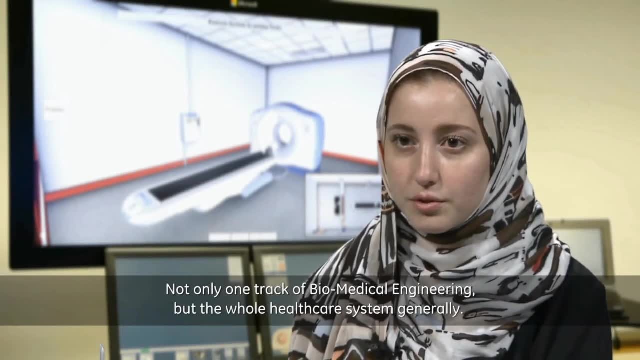 It's a unique training program. We're focusing on everything, not only one track of biomedical engineering, but on the health care system in Germany. So no, I can't wait. We'll be back in two weeks. imagine like what my future can be.